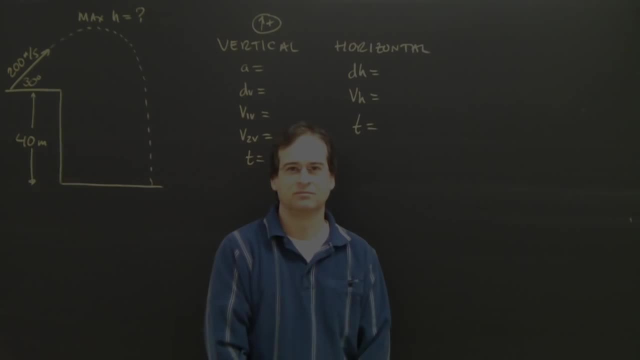 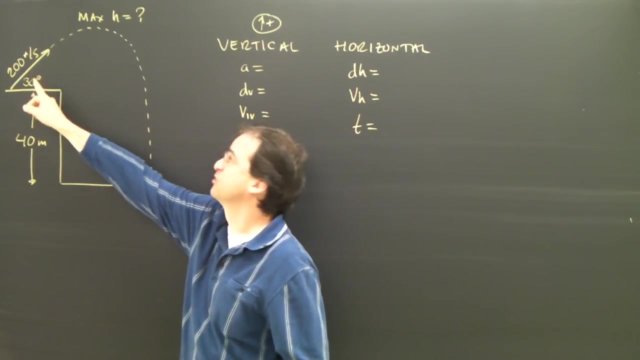 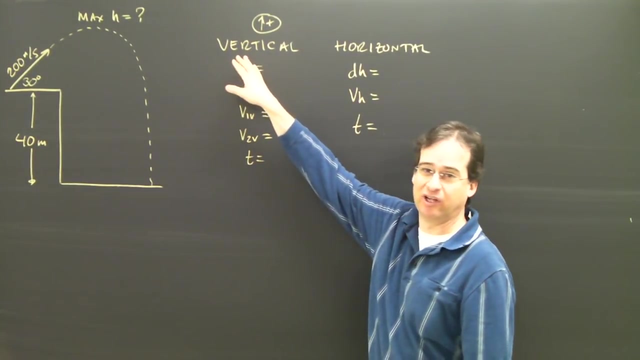 In this projectile problem. what we're looking for is, when we project something off of a building at 200 meters per second, what's the maximum height it's going to travel? Now, when we've done projectile problems in the past, we said we'd look at the vertical column and the horizontal column. 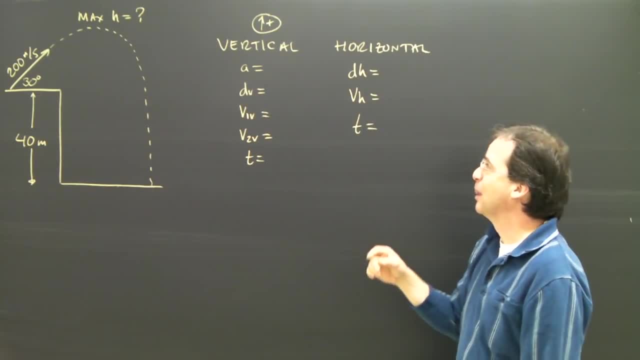 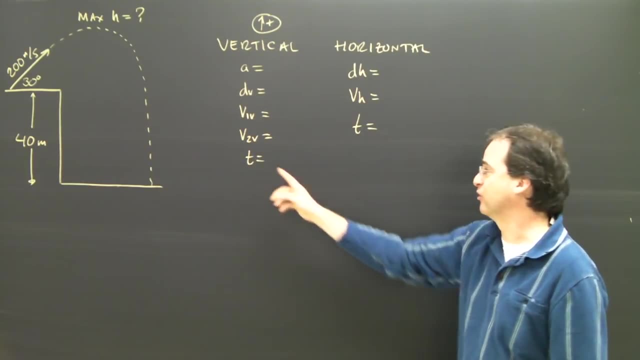 So if you're not sure what I mean by this, check one of the previous videos. But the idea is I put all my vertical information here, all my horizontal information here, and the only thing that can go from one column to another is the time. 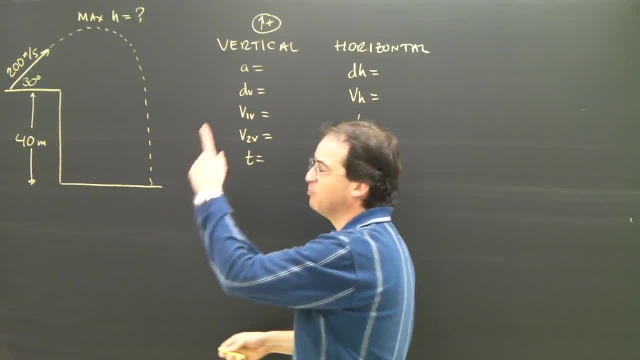 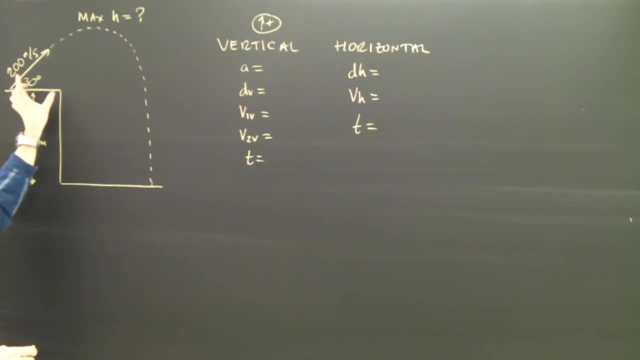 Now, I may not need that in this case, So let's put down our information. We're mostly interested in the vertical. What we have to realize is, when a projectile goes up, its horizontal component will always stay the same, but its vertical component will change. 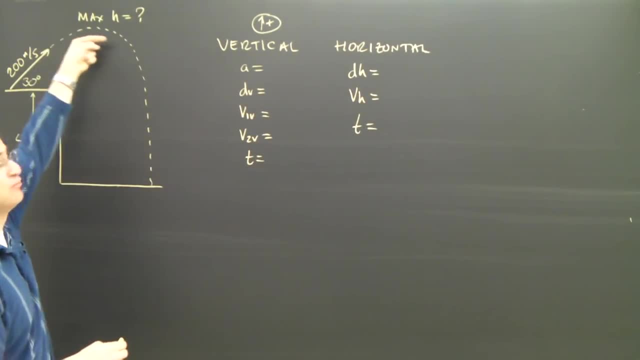 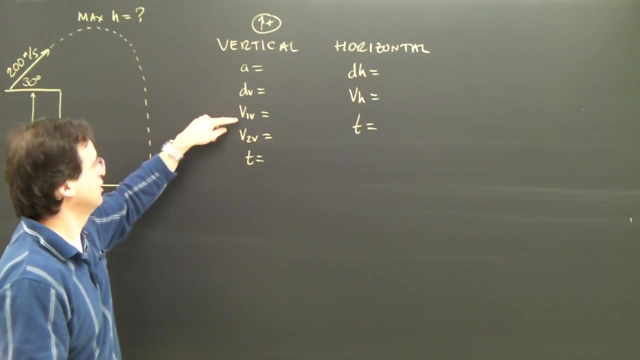 When it reaches its maximum height, it's still moving forward, but its vertical velocity at that point is zero. So at the maximum height, the vertical velocity V2 vertical, the final vertical velocity is zero. So at the maximum height, the vertical velocity V2 vertical, the final vertical velocity is zero. 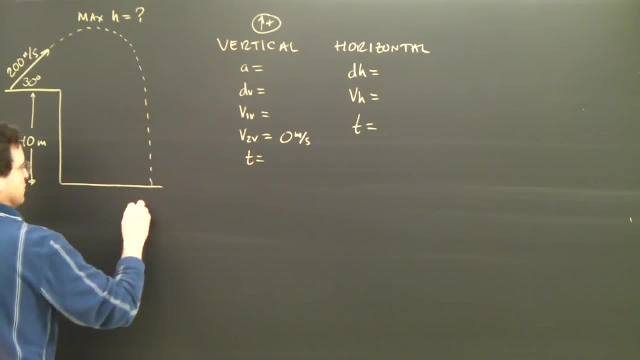 So at the maximum height the vertical velocity- V2 vertical- the final vertical velocity is zero. At maximum H, V2 vertical equals zero. So I'm really not interested in this 40 meters. I'm really interested in what happens from here up to the top. 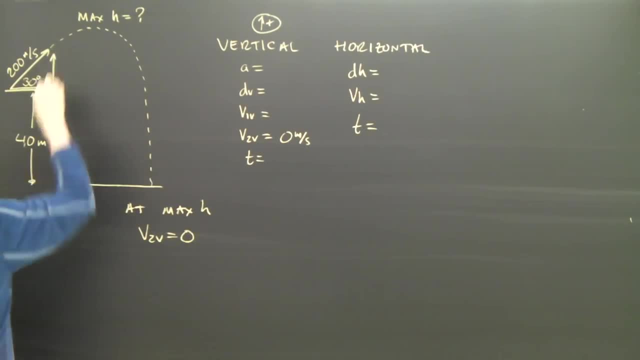 So I have to split this into components. This vertical component is 200 times the sine of 30, which equals 100 meters per second. So even though it's being multiplied, projected at 200 meters per second, that way the initial vertical velocity is 100. 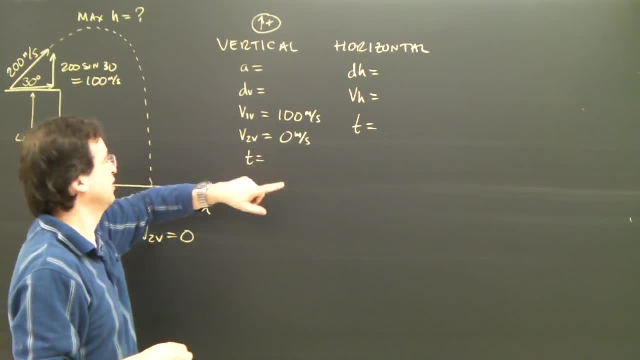 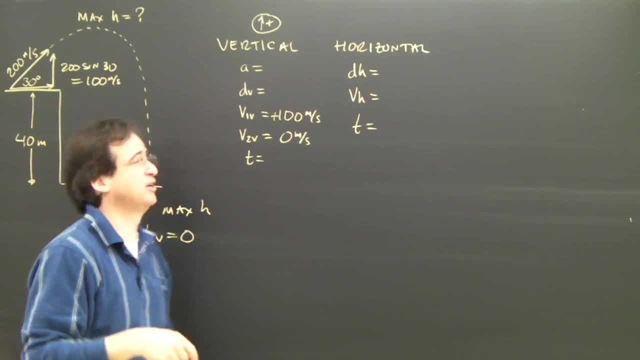 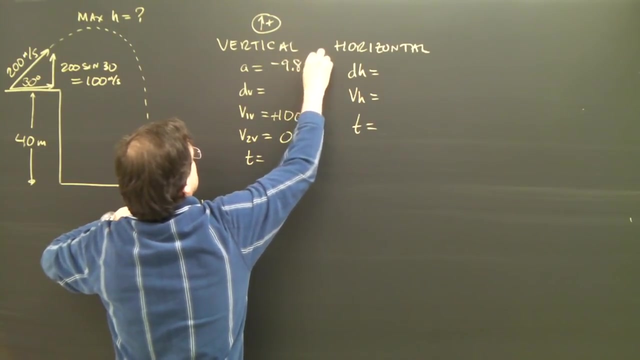 meters per second and I've chosen up as positive. so this is up, it's positive. when it gets to the top it will still be moving sideways, but the vertical component is zero. we know that the acceleration here is negative. nine point eight meters per second square. I now have three of my variable, so now I can.